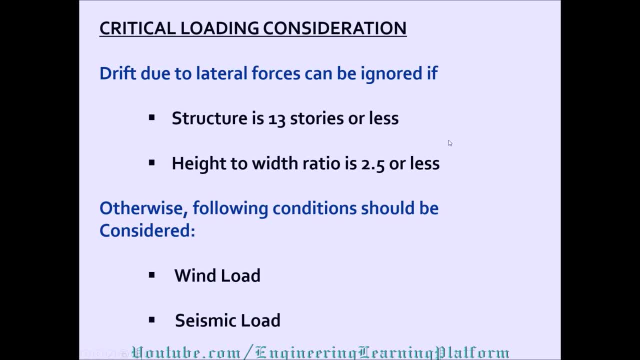 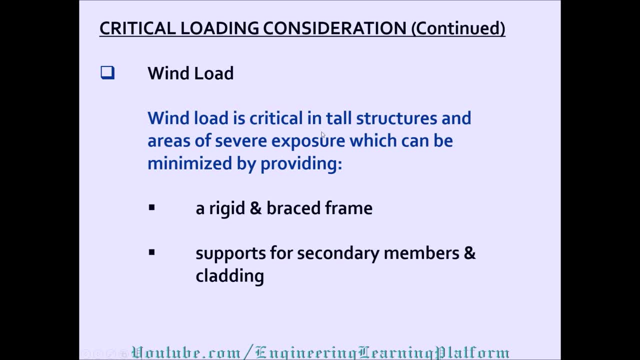 be considered. This is not recommended in any code, but this is what I am telling from experience working in design office. Wind load is a critical load in tall structures and areas of severe exposure can be minimized by providing a rigid and braced frame Supports. 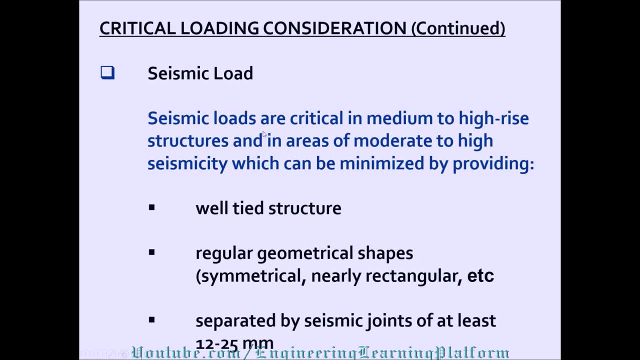 for secondary members and cladding. Seismic loads are critical in medium to high rise structures and in areas of moderate to high seismicity, which can be minimized by providing well-tied structure or you can say braced structure or different kinds of structural systems utilized in tall structures. Regular geometrical shape is not recommended in the 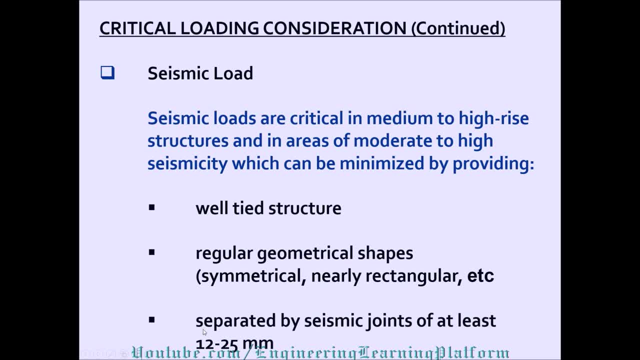 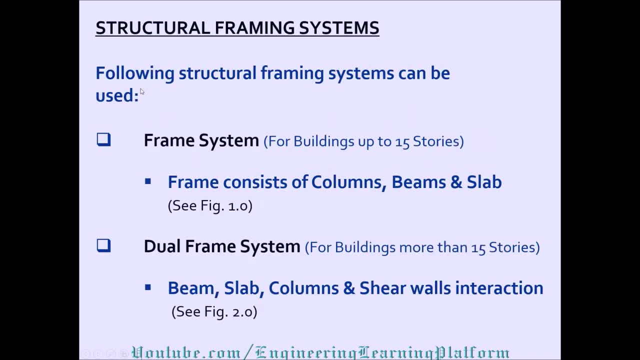 shape: symmetrical, nearly rectangular, etc. separated by seismic joints of at least 12 to 25 mm. Following structural framing systems can be used: Frame system for buildings up to 15 storeys. Frame consists of columns, beams and slab. 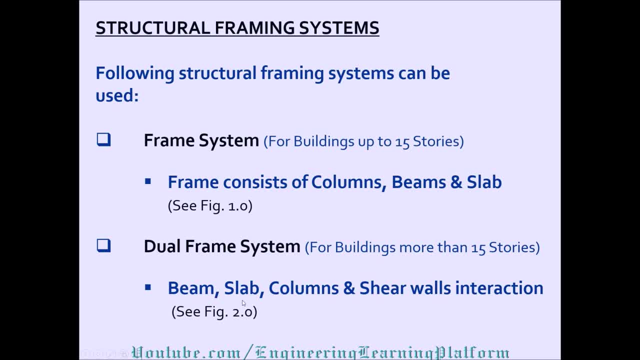 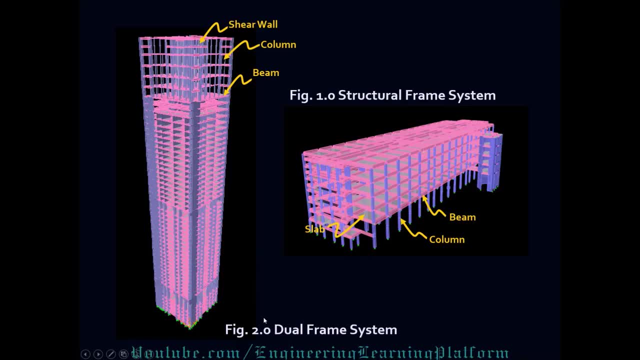 Dual frame system for buildings of more than 15 storeys: Beam, slab, column, shear walls interaction. The figures will be shown shortly. This is why figure number 2, it shows shear wall, column, beam and similarly this is: 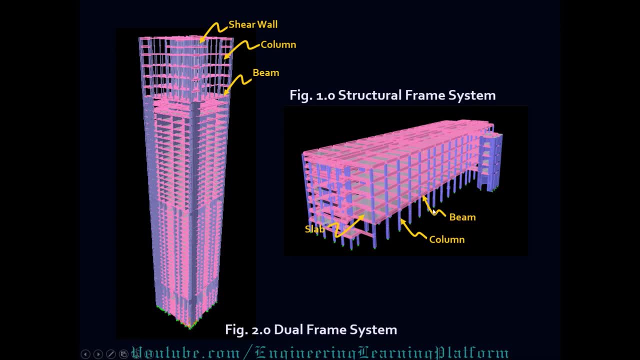 a structure which has a lesser height and a higher width, The beams, columns. slab Beam is referred as a structural member in which the axial load is less than 10 times of Agfc prime, While column is a structural load in which the 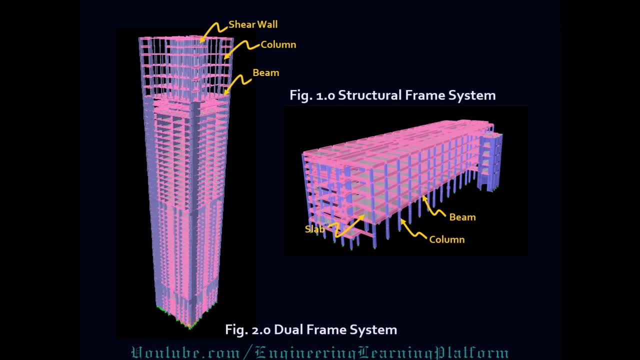 axial load is less than 10 times of Agfc prime. While column is a structural load in which the axial load is less than 10 times of Agfc prime, The axial force is greater than Agfc prime divided by 10 according to ACI code. 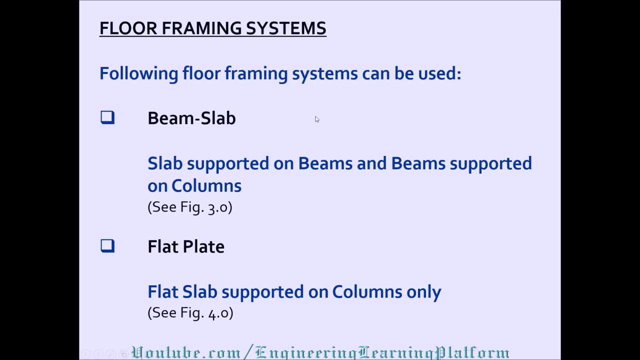 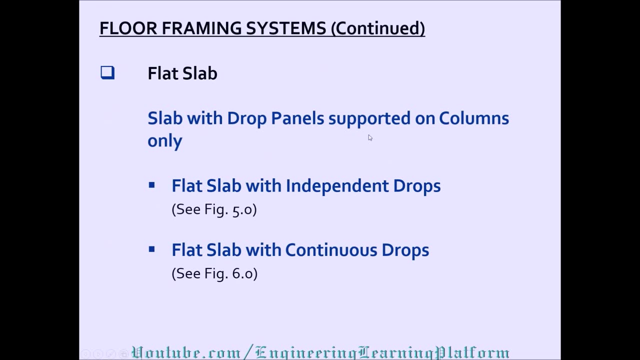 Floor framing systems. Following floor framing systems can be used: Beam slab system Slab supported on beams and beams supported on columns. Flat plate system- Flat slab supported on columns only. Flat slab Slab with drop panels supported on columns only. 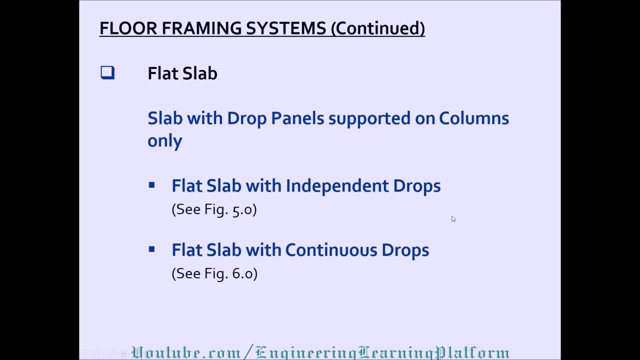 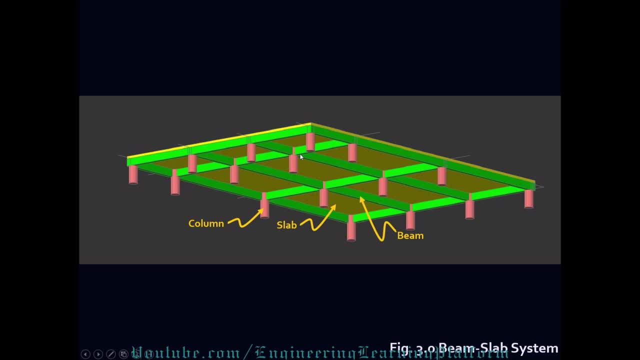 Flat slab with independent drop panels only. Flat slab with continuous drops. Flat slab with continuous drops. This is a beam slab system in which the columns are first connected to the beam and then connected to the slab. There is no punching shear required in the beam slab system. 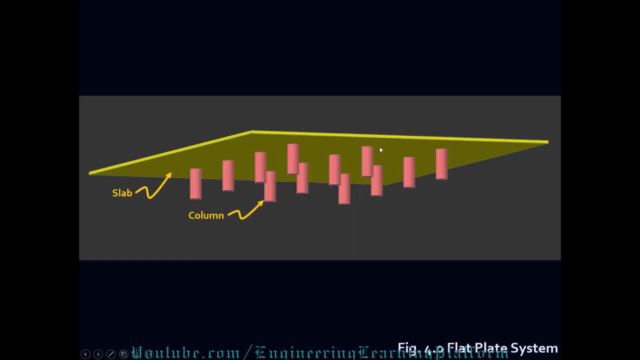 While this is a flat plate system, it doesn't have any beams, as well as any drop panels or column capitals at the intersection of slab and columns- columns- so the punching shear is very critical, and these slabs end up having higher thickness compared to gleam slab system. this is a very ideal system for 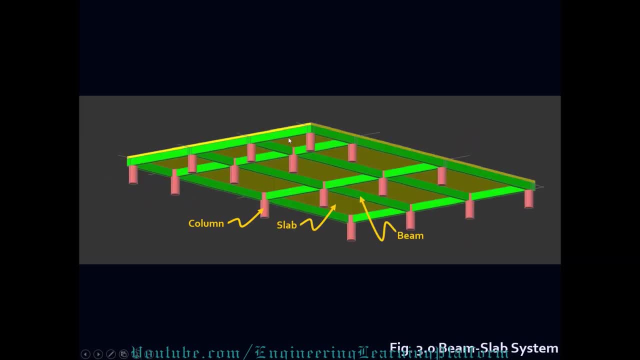 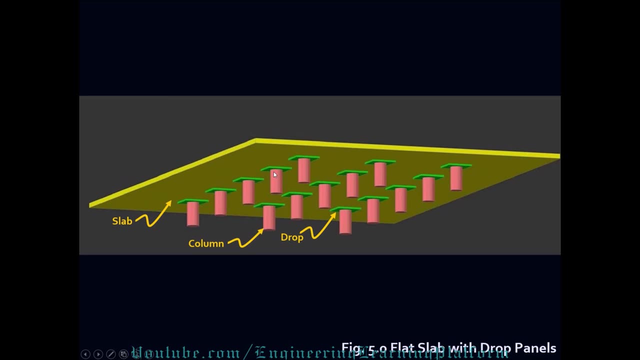 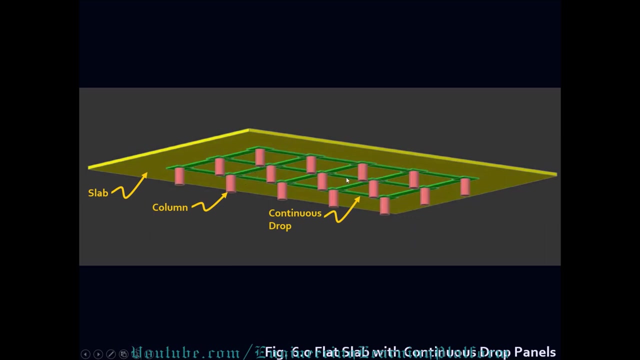 parkings, where we need headway or clear headways. while this is a very ideal system for residential floors or office floors with partition walls, this is the flat slab system with column capitals or drop panels. this is called a drop, this is called a continuous drop. when the one-way shear is very high, then we 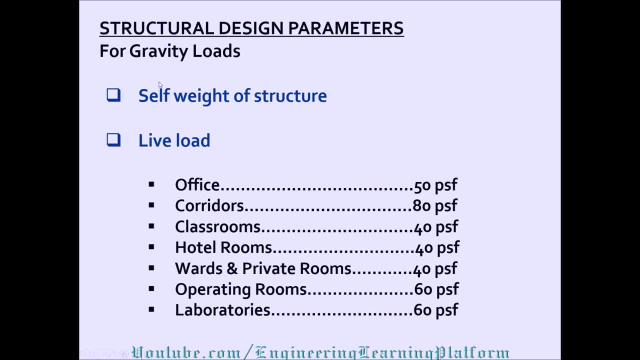 provide continuous drop. structural design parameters for gravity load. important parameters for gravity load are: self weight of the structure. live load. live loads according to UBC 97 is 50 PSF, for corridors 80 PSF. it depends upon the occupancy of structure: classrooms: 40 PSF. hotel rooms 40 wards and private rooms 40. operating room 60. 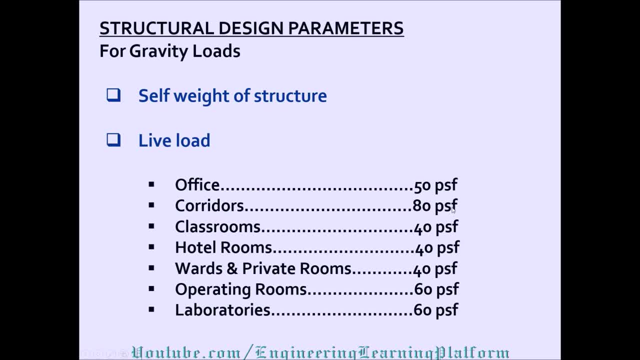 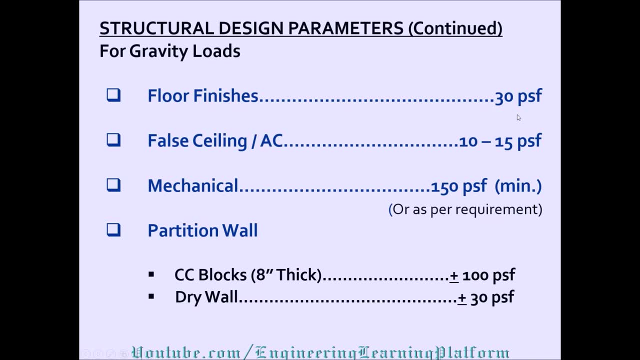 and laboratories: 60 PSF. PSF refers to pound per square feet. this is according to American codes. floor finishes: 30 PSF if it is of 2.5 inches false ceiling AC. these are typical dead loads. floor finishes: 30 PSF if it is of 2.5 inches false ceiling AC. these are typical dead loads. 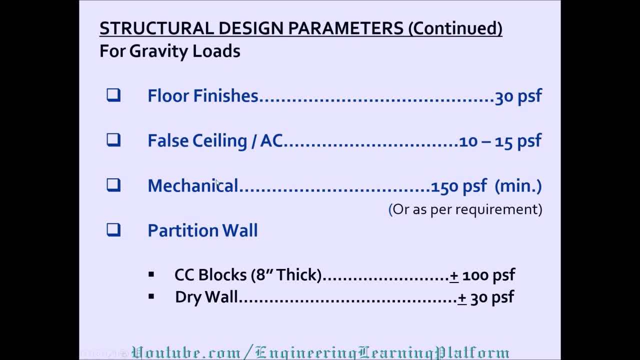 mechanical 150 PSF minimum or as per requirement. this is heavy mechanical load. there is another category of heavy mechanical load that refers to 200 or even 400 PSF. that can be calculated easily if the mechanical or HVAC equipment floorplan is provided. partition wall consists of CC blocks 8. 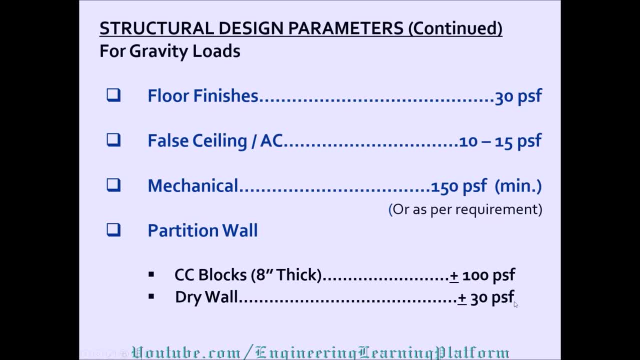 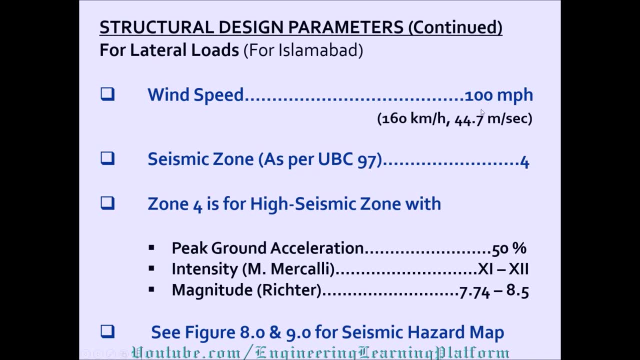 inch thick, then the load is 100 PSF plus minus and the drive-all is 30 PSF. wind speed is 100 PSF plus minus and the drywall is 30 PSF. wind speed is 100 miles per hour in most part of Asian countries. seismic low zone aspect- UBC 97. 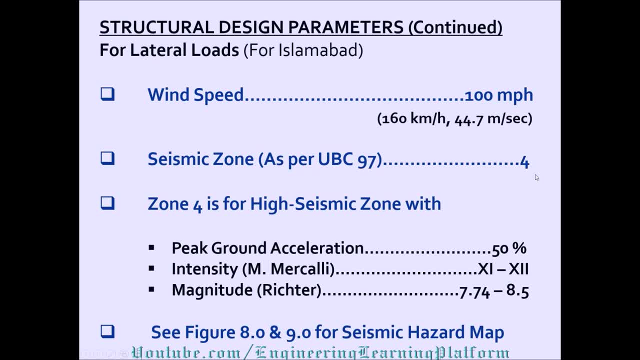 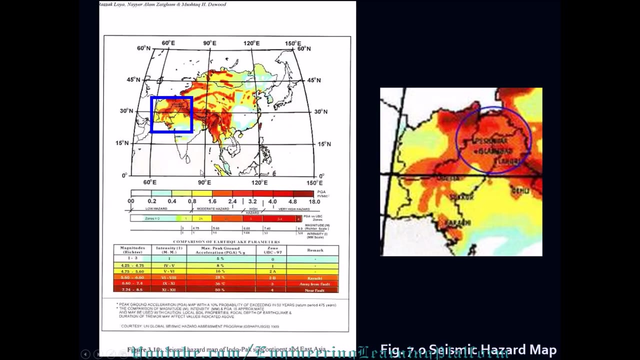 is classified as 1 to 2, a to be 3 and 4. zone 4 is high seismic zone. peak ground acceleration is 50%. intensity ranges between 1 to 10 or 9 in some cases, while magnitude is richer scale. the seismic hazard map looks similar to the one. 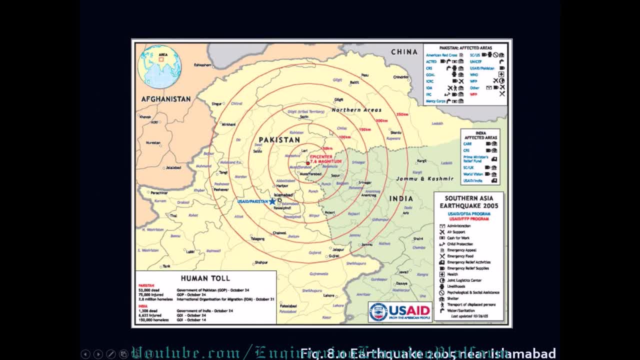 shown on the screen and, for example, this seismic hazard map is for Pakistan and this is the epicenter having magnet maximum magnitude of 7.6 earthquake. the magnitude is classified as one value for the earthquake, while the incentive intensity of earthquake varies as a distance increases with the earth from the earthquake epicenter. intensity at 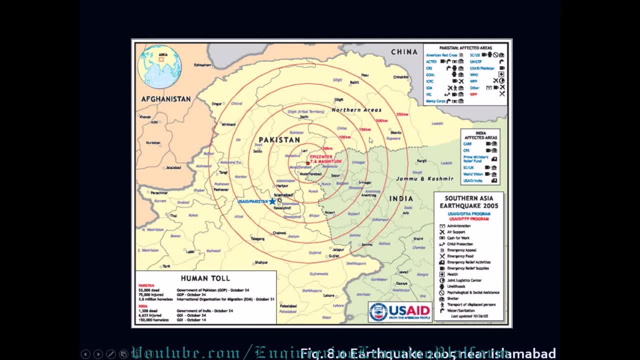 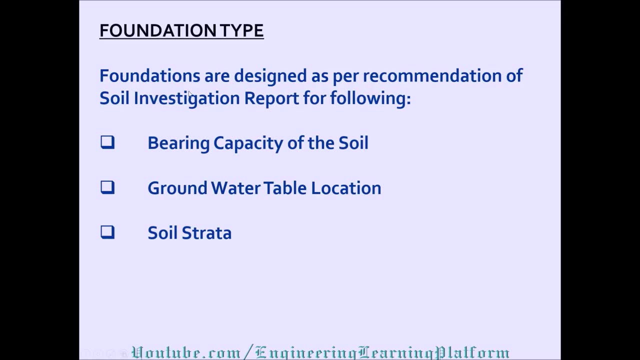 epicenter is equal to magnitude, while the intensity of earthquake decreases with increase in distance from the epicenter of earthquake. epicenter is defined as a point from where earthquake is generated. foundations are designed, as per recommendation of the soil investigation report, of the following: bearing capacity of soil, groundwater table location, soil strata. on this basis, 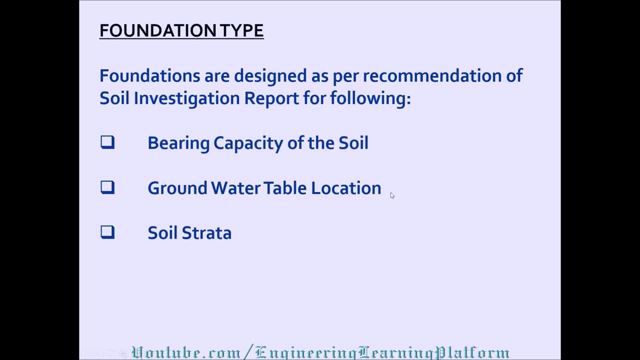 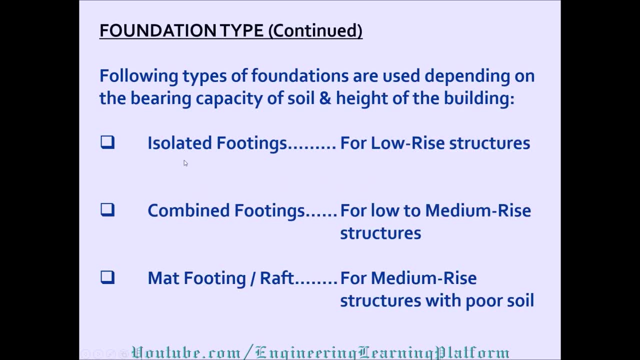 we select what kind of structure would be having, whether it should be having deep foundation or shallow foundation. the foundation can be consisting of isolated footings for low rise structures, combined footing for low to medium rise structures made, or raft footing for medium to high rise structure with. 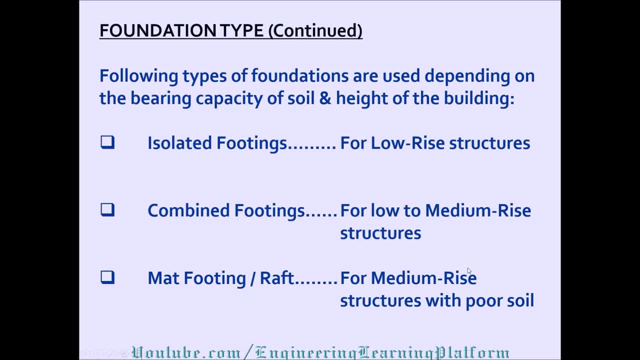 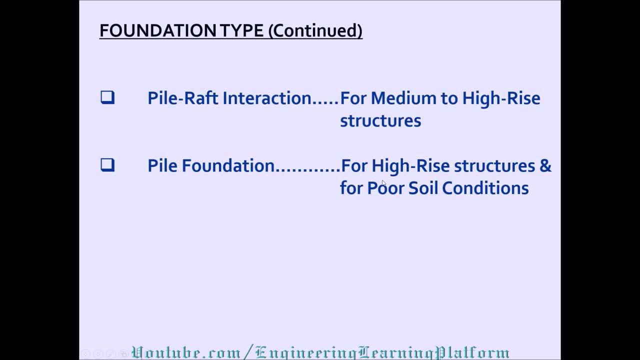 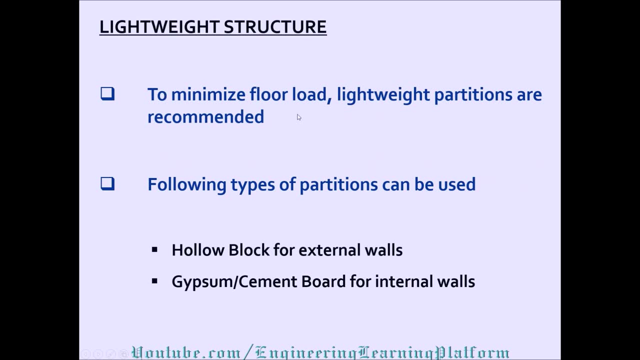 poor soil. it is also some cases medium rise structure. appropriate pile and raft interaction for medium to high rise structures. pile foundation for high rise structures for work soil conditions. lightweight structure: to minimize the low flow load, lightweight partitions are recommended. following types of part divisions can be used: hollow block for external walls. gypsum cement board for 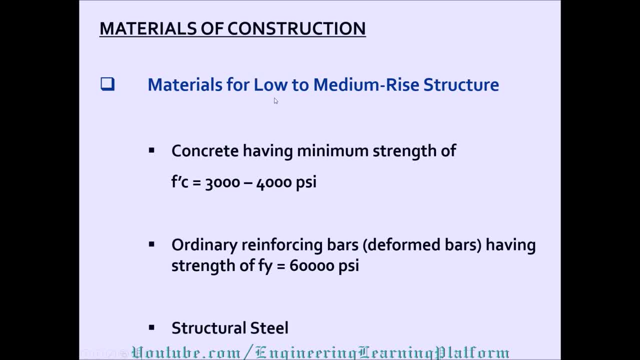 internal walls. materials of construction can be used as follows. the following types of partitions can be used: hollow block for external walls. gypsum cement board for internal walls. materials of construction for loa to mitrise structure concrete having people having minimum strength of 3000 to 4000 psi. ordinary rain spursing bars. 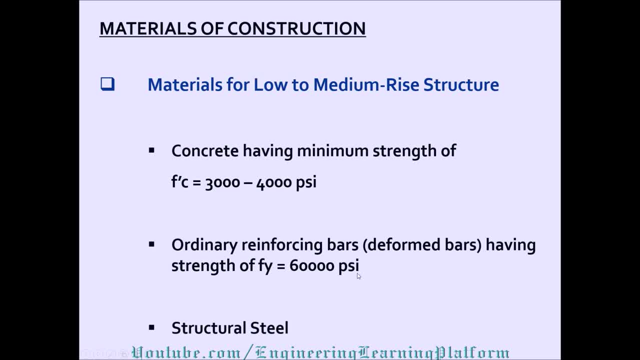 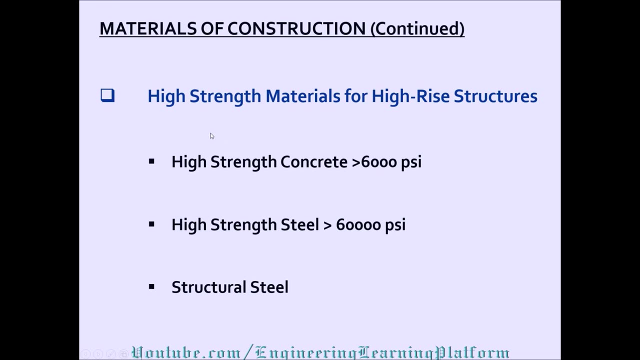 deform bars having strength of yield strength of 60,000 psi, and then we have a structural steel buildings ranging from 36 ksi is天thu 50оля, and then we have high値 grades of concrete. the high성 station, USD location, grows creation works during construction, group facilities, local & local development. construction for low to mid rise structure concrete has in whole sala. construction for low to majorized structure concrete, effective met hair players, ordinary bar's, deformed bars and characters having strength of yield. presidente suggest cranelistic performance. and then we have structure building粵 е reviewVoiceover a matter of 50 KSI. and then we have high matic rates of concrete, the highắmodysery milk & 내. 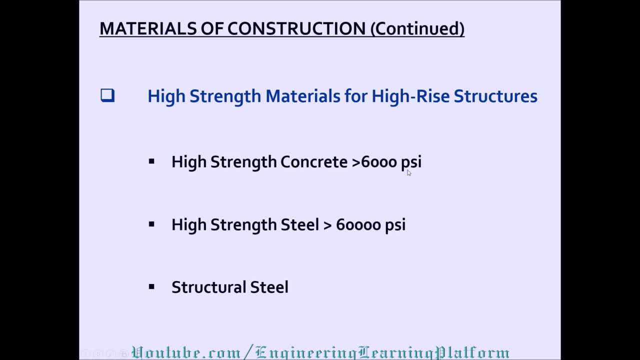 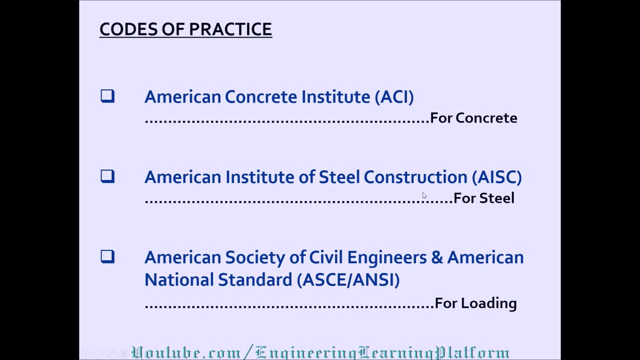 material for high rise structure can be greater than 6,000 psi. high strength steel can be greater than of 60,000 psi strength. then we have structural steel, codes of practice, American Concrete Institute for concrete, American Institute of Steel Structure for steel. then we have American Society of Civil Engineers and National Standards. 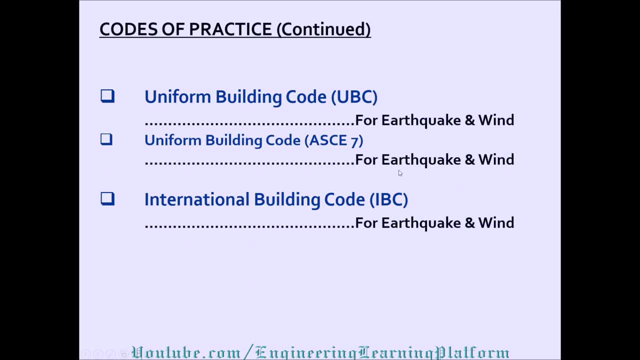 ASCE and ANSI is for loading. we have Uniform Building Code for earthquake and wind load and Uniform Building Code as well, referred as ASCE-7, which is an upgraded version of UBC and IBC code. then we have International Building Code IBC, for earthquake and wind load. 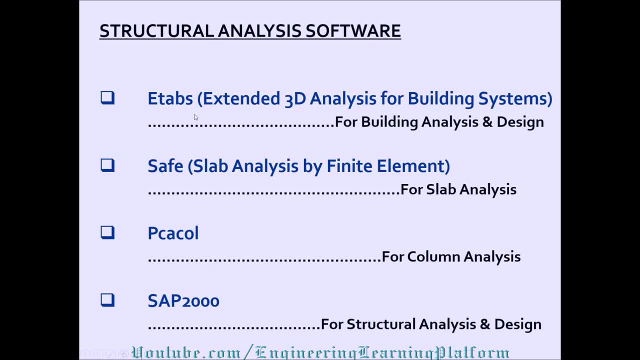 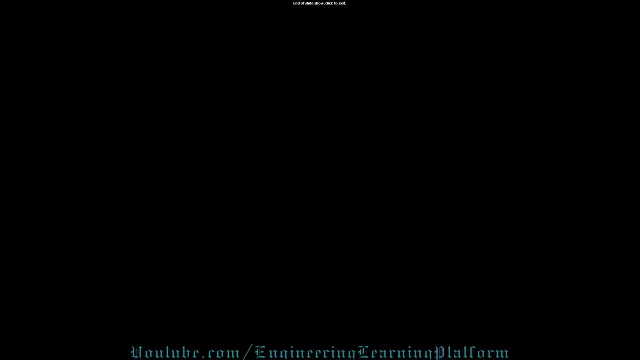 the structural analysis software we have ETAPS, SAFE, PCA-CALL, SAP2000. ETAPS is used for building analysis and design. SAFE is utilized for slab analysis as well as foundation analysis. PCA-CALL is used for detailed column analysis, SAP2000 for structural analysis and design of miscellaneous structures such as steel structures. 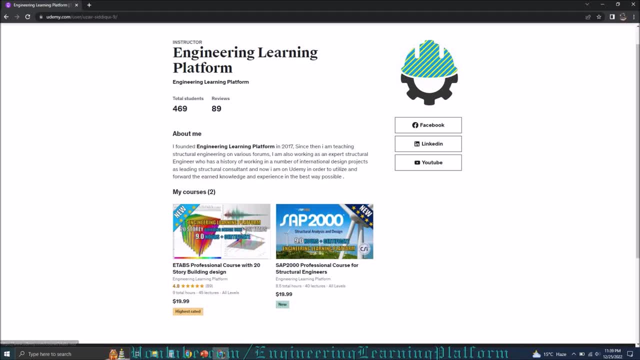 if you are interested in structural engineering, then I would highly recommend you to attend ETAPS professional course, with a 20 story complete design of building, as well as SAP2000 professional course, which covers the aspects of structure analysis and design using SAP2000, from basics to advanced level. 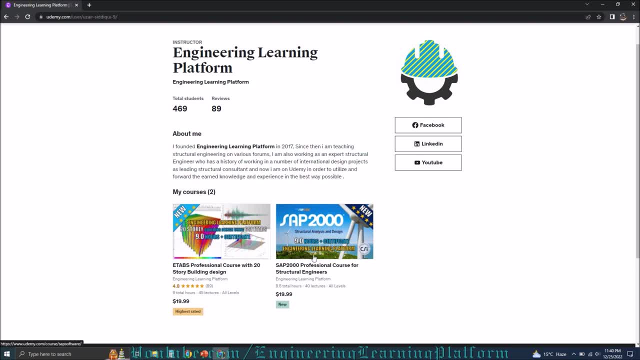 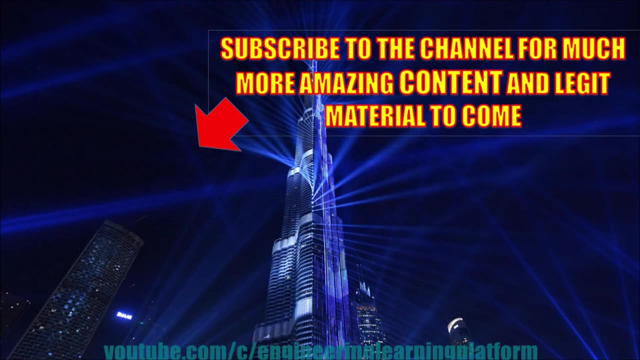 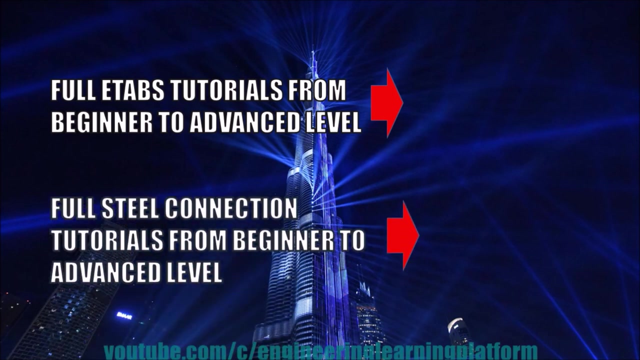 if you are looking for a career in structural engineering, you must look at the courses published at UDEM. the link to these courses is given in description of this video. thank you for watching wwwsap2000.com.